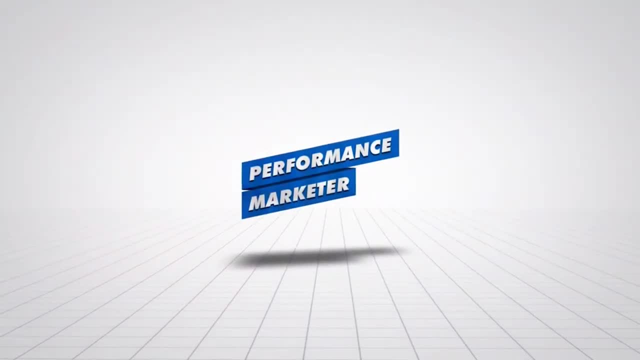 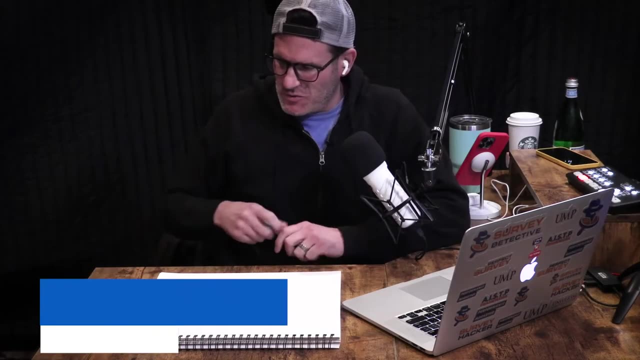 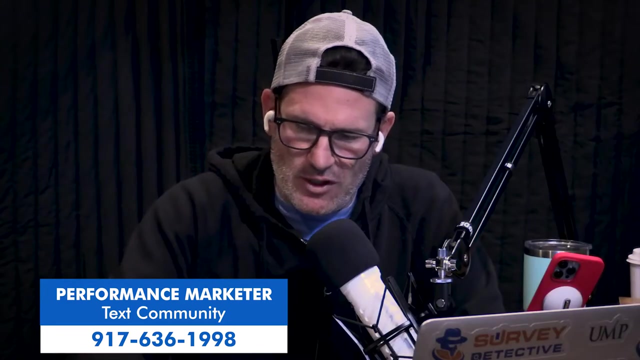 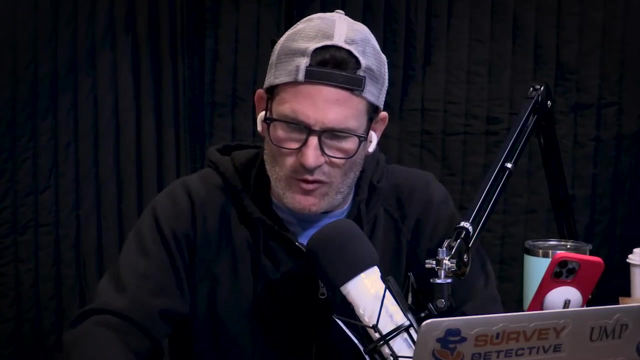 How my mind thinks about this and then you can work with me here. But I just want to, you know, be really simple on what's going on. So if you look at when someone's buying traffic, okay, you have the whole internet and that's got traffic all over the world. 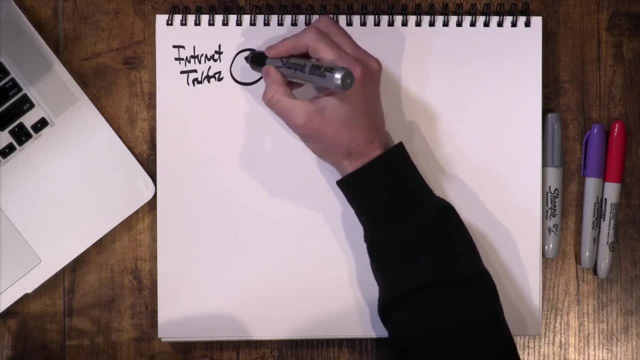 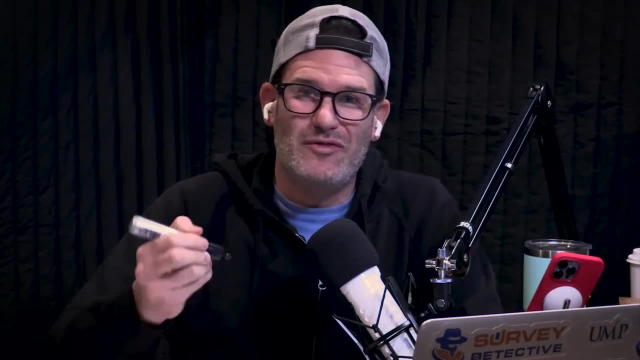 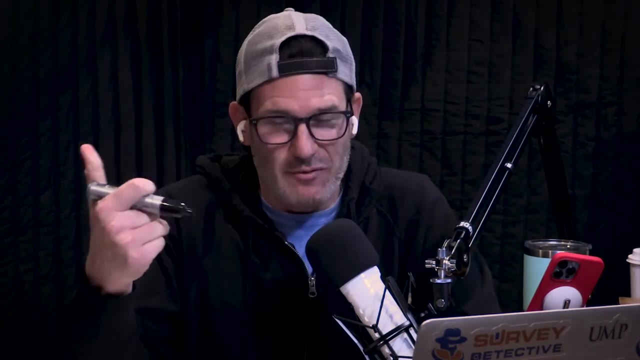 All over the world. So here's a globe right with, like all these different cities and states- and I'm not an artist, right, So we know that we're looking for a certain person when we're out in the marketplace And the way we buy traffic is right. we talked about this First. 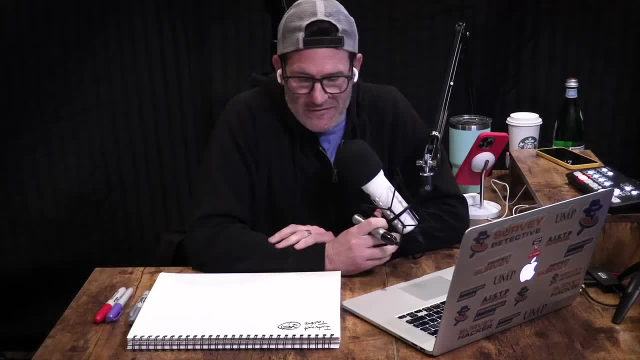 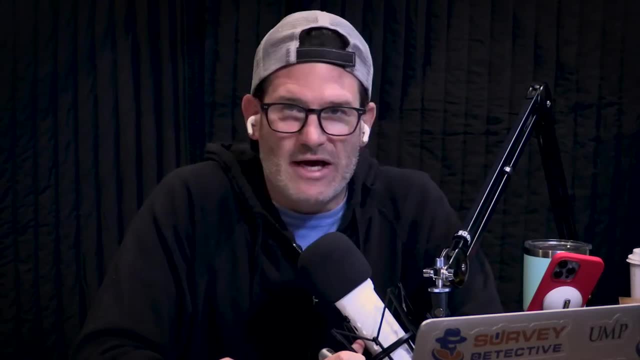 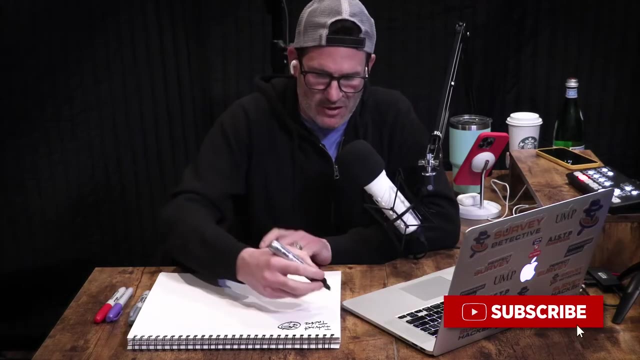 who are we talking to, right? Who are we looking for? Then we got to figure out where they are in the internet, And once we can identify where they're hanging out now, we got to go back and grab their attention, right. We got to start to create some ads and then buy traffic, right. 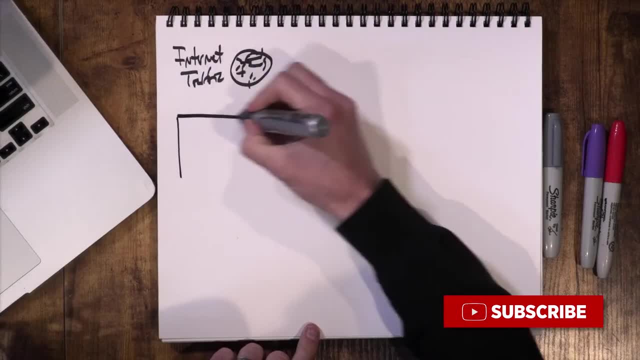 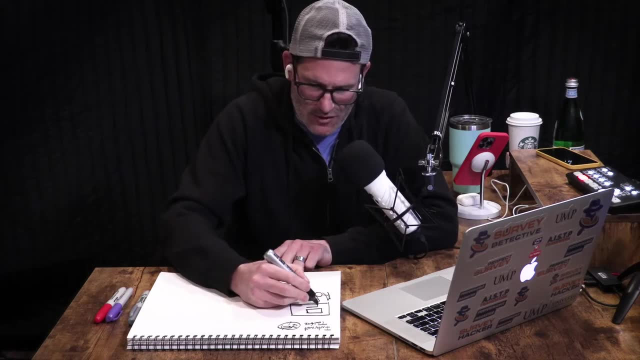 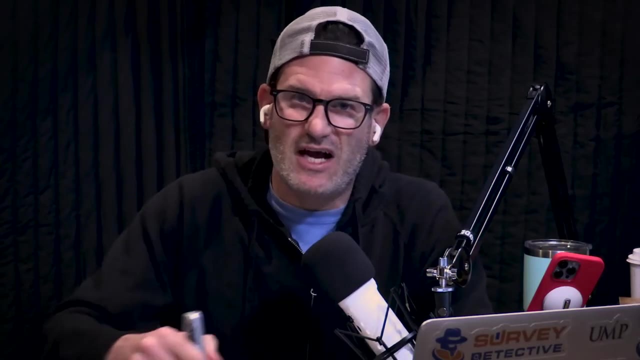 So we create ads. right. So here's an ad. right, So maybe it's a video with a click here, right? So what we're doing here is we're creating all different kinds of ads because this is the ad, all right, This is the ultimately attracting. 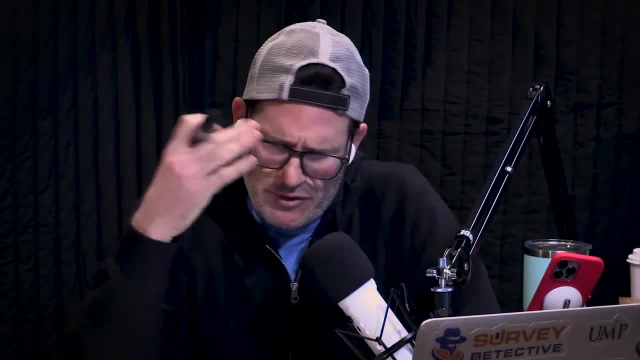 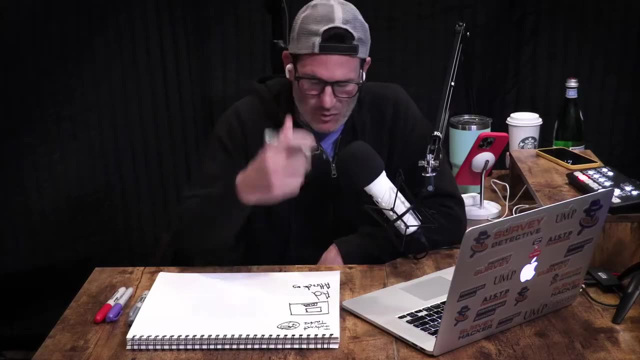 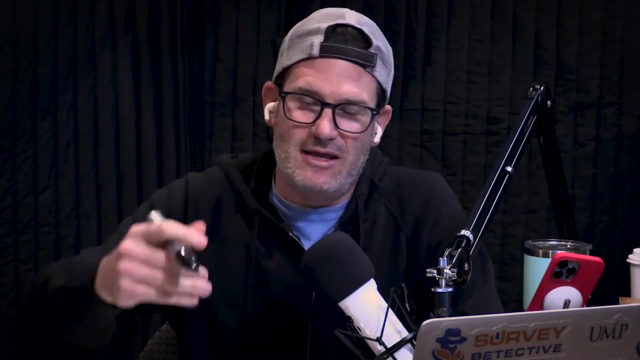 Right, We're attracting somebody. right When we talk about the AISTP. right, Amazon is selling toilet paper, AISTP, we're attracting people with this. right, We're trying to create a pattern, interruption. right, We're trying to get somebody to say: you know, whoa, what is that? right We're 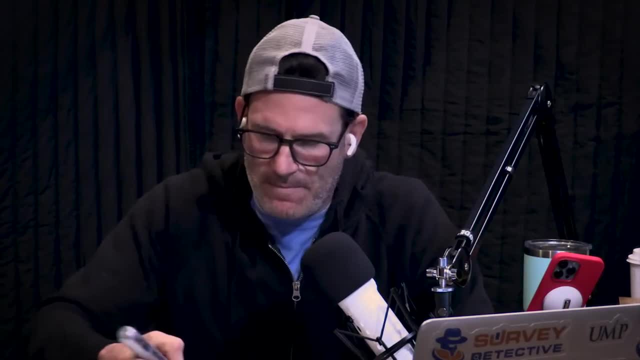 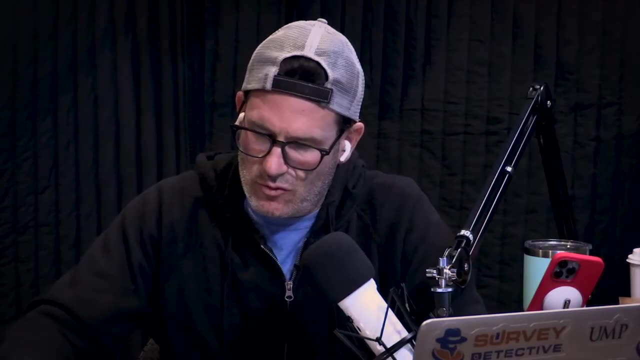 trying to create some curiosity, right. So somebody clicks. We get somebody to click. Now we're sending them a message. We're sending them a message. We're sending them a message. We're sending them to a destination of our choice, right Our landing page, And in this, 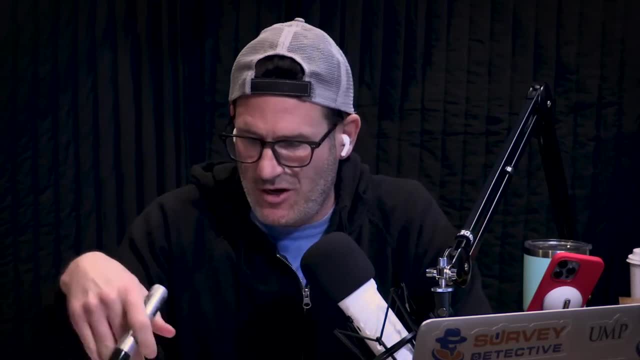 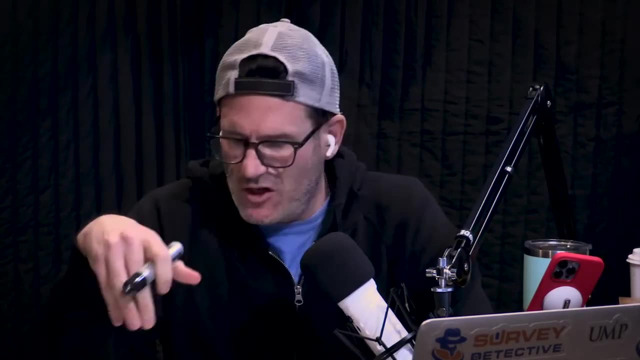 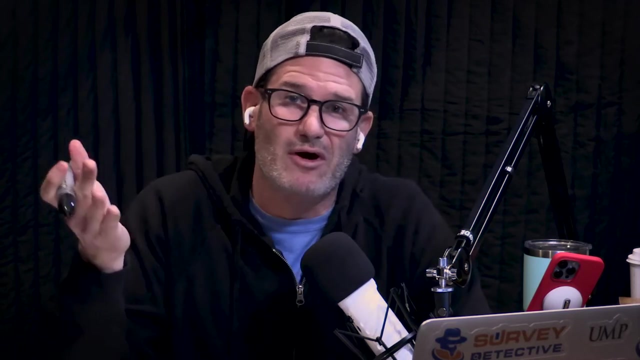 scenario. this could be a number of things, right. It could be a content page, It could be a lead form, It could be, you know, just an interstitial page, a video page You could send them to. you're subscribing to YouTube, right, Which is where we are right now. So, you know, maybe you're. 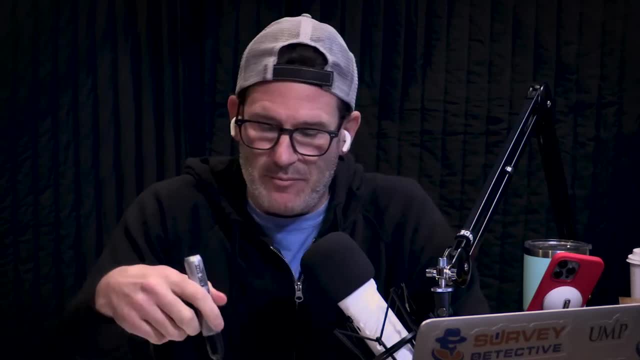 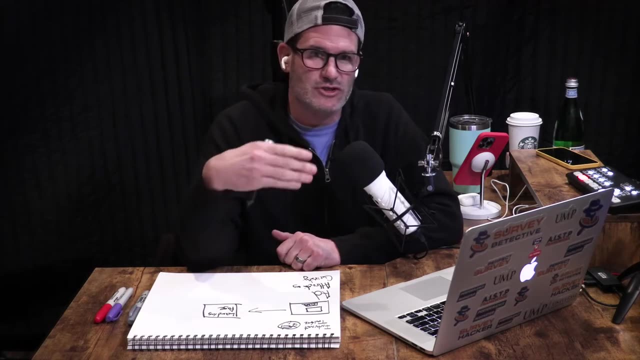 here from us getting you to subscribe to my channel By buying an ad. you then clicking, doing something. maybe you took a survey and at the end of it, the goal was to try to get you to subscribe to my YouTube channel. So you know if you went. 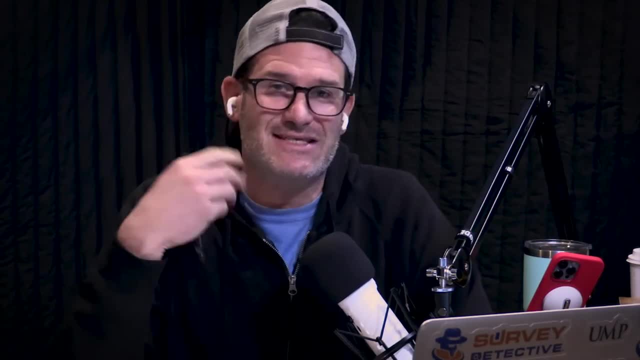 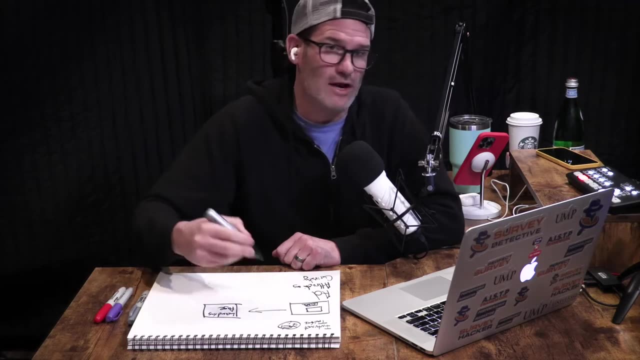 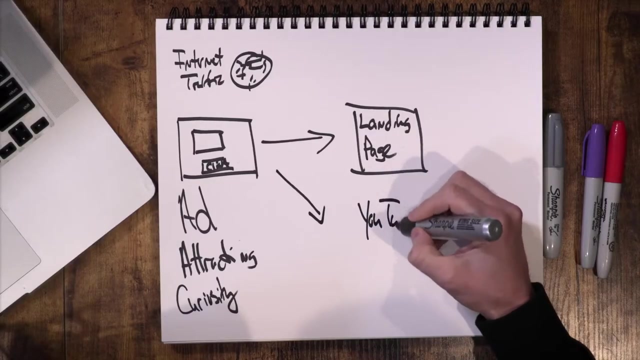 through that, then awesome, I'm happy you're here, right. But that's the concept, right? It could be a simple: you know, subscribe to my YouTube channel, a little teaser here, click and then go right to my YouTube channel, right? So in that scenario, that would be to YouTube's right. 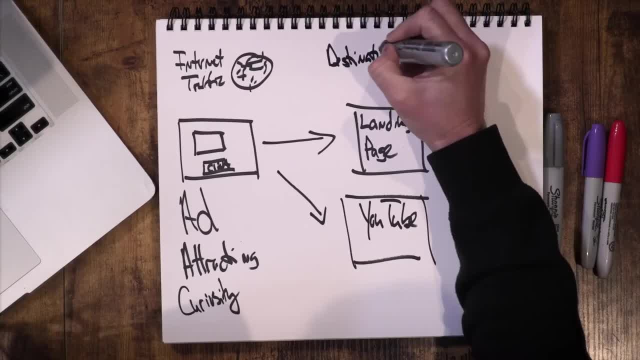 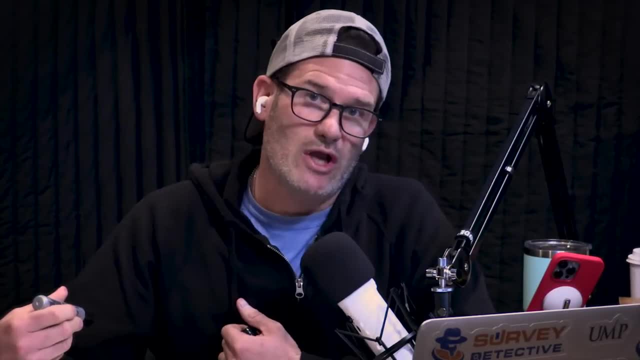 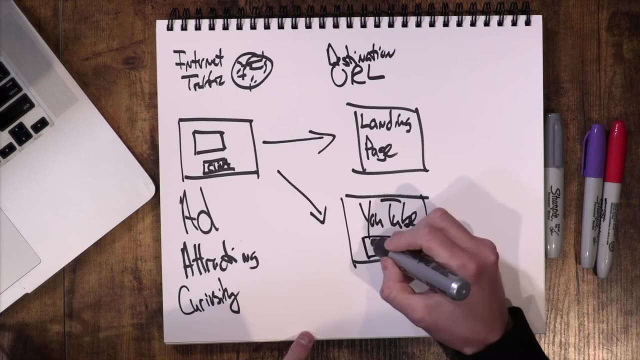 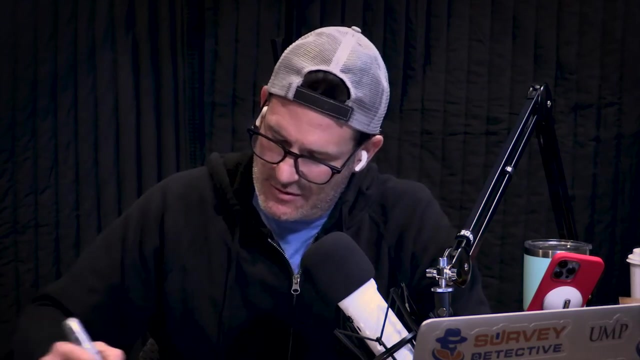 So this is the destination URL, right? So in this scenario, we could be sending somebody to a landing page which we own to capture data, or we could be sending them to YouTube to get them to subscribe- right, They could send them to my podcast Again to subscribe. 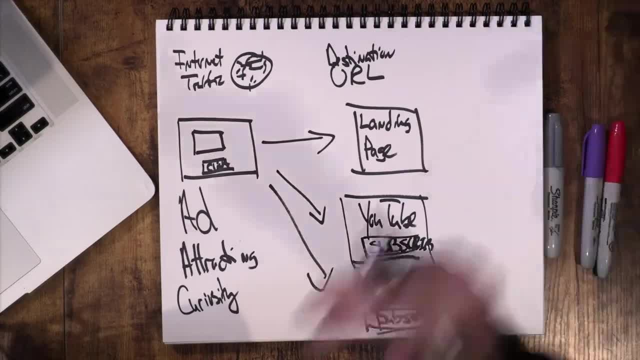 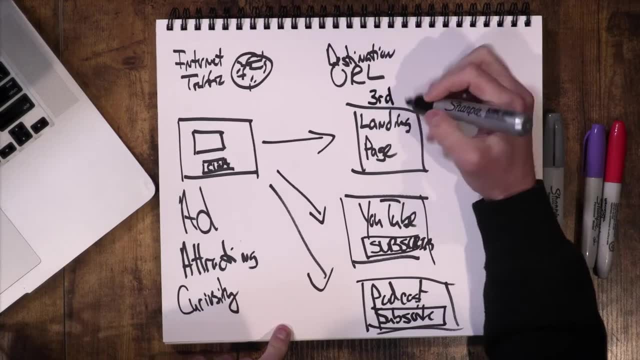 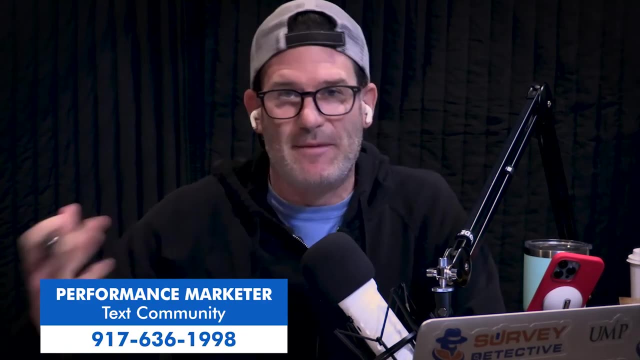 I only own this page right here, right, An affiliate, right? Somebody who's an affiliate can send something to a third-party landing page, right, Third-party? So if I own an offer, I can give it to somebody to drive traffic to my page and then I pay them on some sort of. 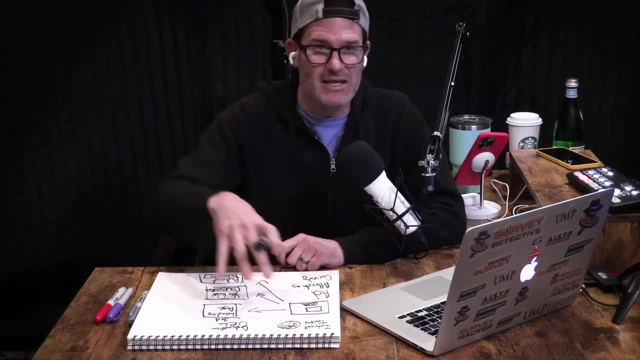 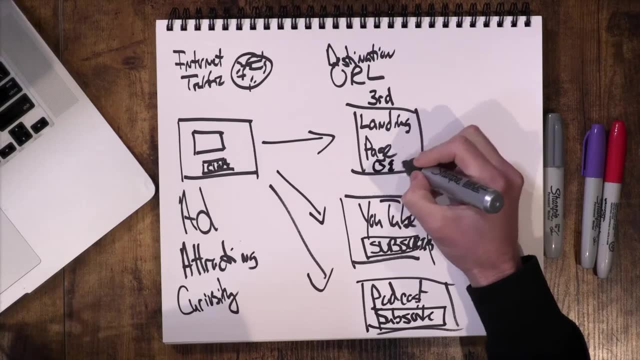 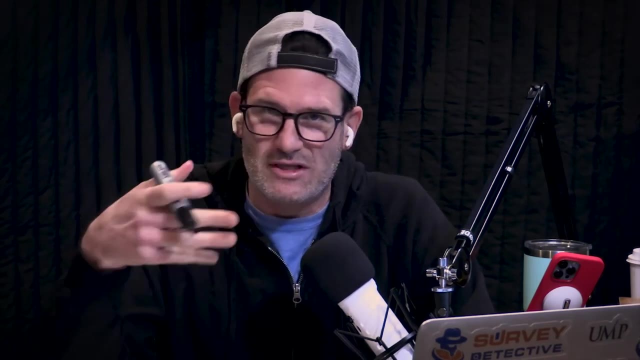 commission. okay, So that's what we're going to look at today- is buying media for ourselves. whether it's going to a third-party landing page or our own owned and operated landing page, right, It doesn't really matter how we're evaluating it, It's all relatively the same. 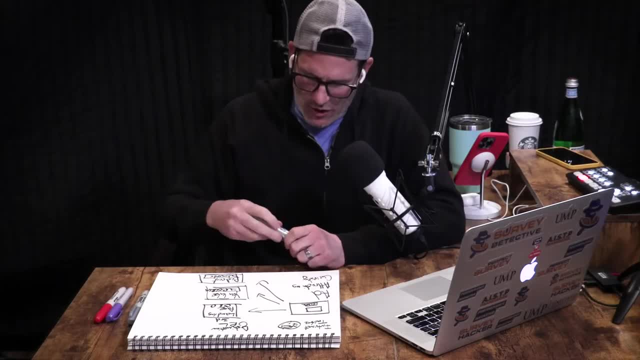 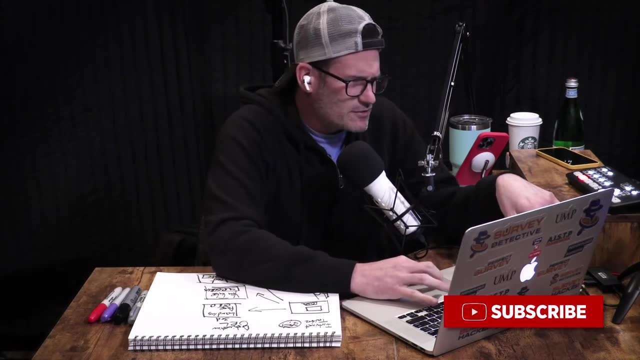 thing, okay, And here is how we're going to do it. So let's go over to this spreadsheet here and take a look, So pretend like we're running a bunch of different offers here, right, And we're looking at clicks, right. So here's. 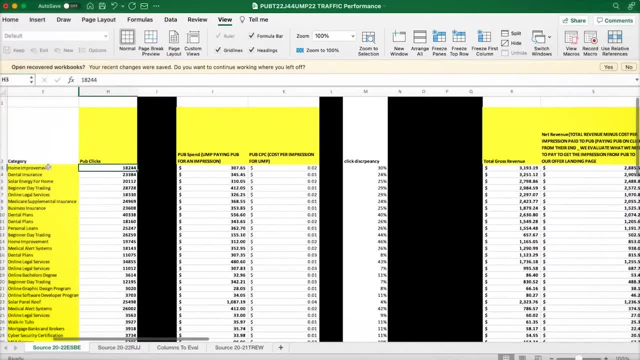 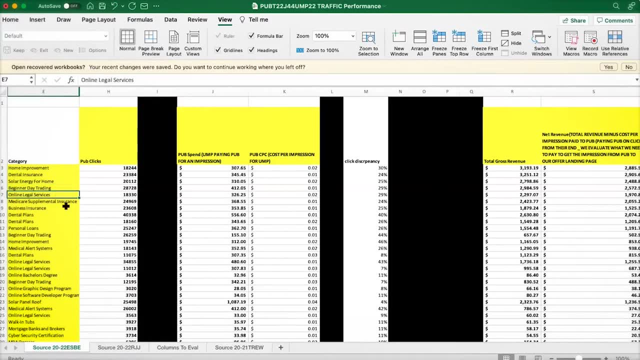 The total clicks. So we're seeing like a home improvement offer, a dental insurance offer, solar energy for homes, beginner day trading, online legal services, Medicare supplemental insurance- right, It doesn't really matter, Like what I'm trying to teach you guys here. 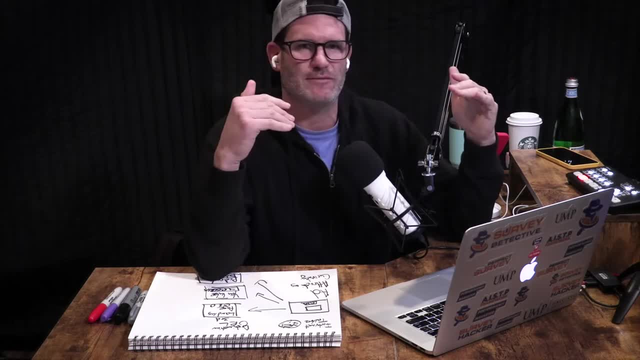 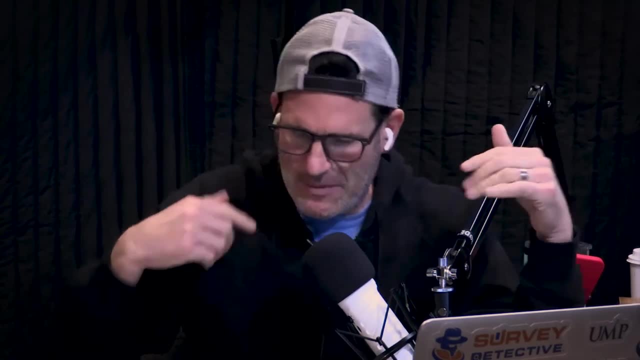 it doesn't matter what you're promoting. I'm trying to teach you something that is evergreen. okay, Everybody know what evergreen means. Raise your hand, Yeah, Okay, It lasts forever. right, Like I don't want to teach you something that you're going to learn. 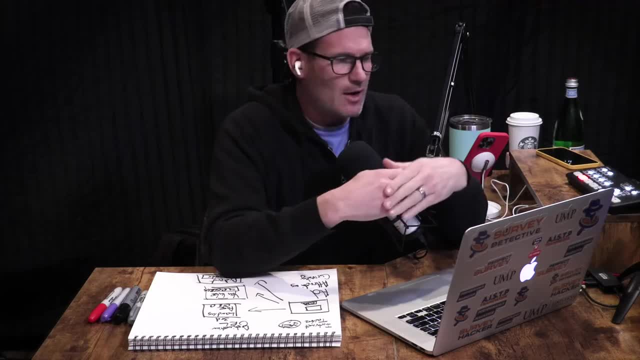 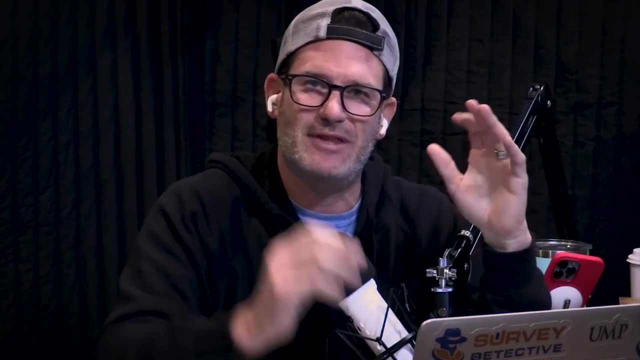 for the next year, and then it's not relevant. I want to teach you something that you can use, no matter where you are on the internet, where you're buying media, And it's the concept, the high level frameworks, the strategy behind all of this that allows you to learn something. 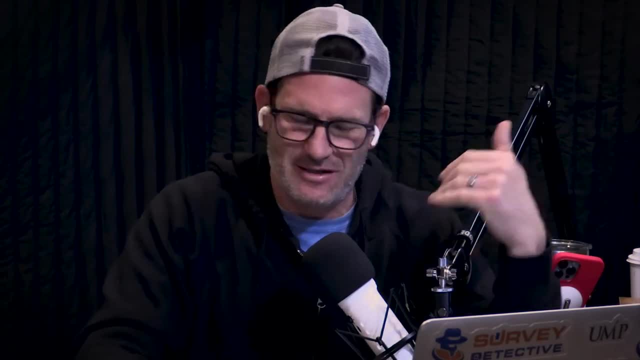 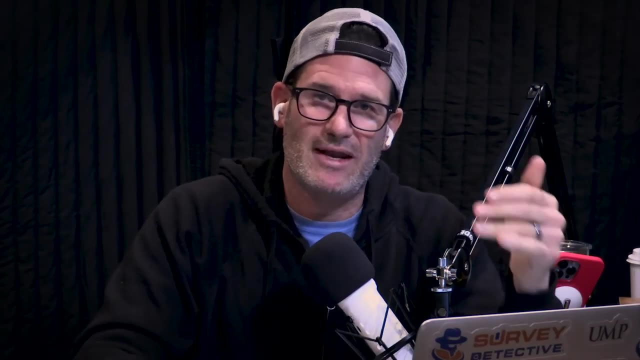 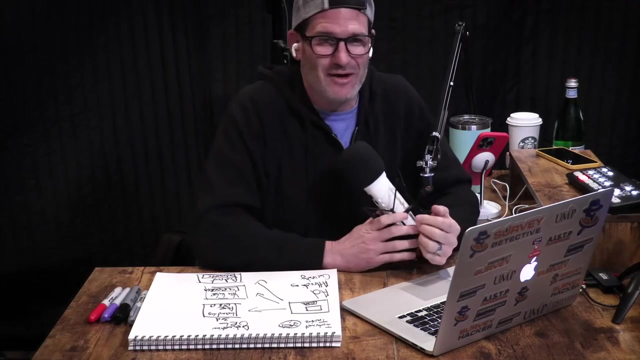 that will last forever. And now it's like: what do they say? Give a man a fish, he eats for the day, Show a man how to fish, he eats for a lifetime. Oh, terrible delivery, Terrible delivery. But hey, you guys, I'm authentic, I am who, I am right, You can tell. 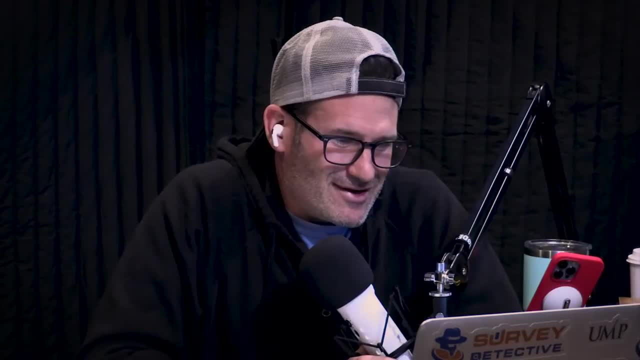 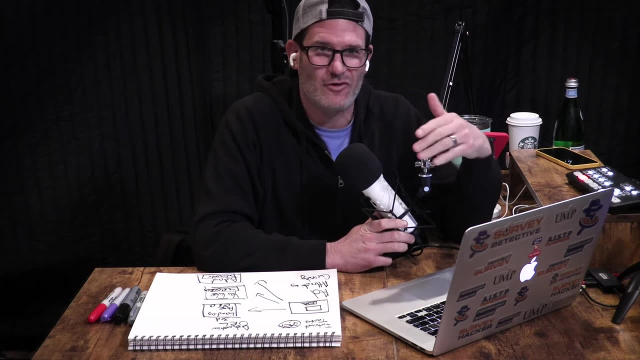 that this isn't scripted. It's just me talking to you guys. But yeah, that's exactly right. So right, It's: teach a woman how to fish and she'll eat for a lifetime. So that's what we're doing here: We're teaching you how to fish, We're teaching you how to find the fish so that you 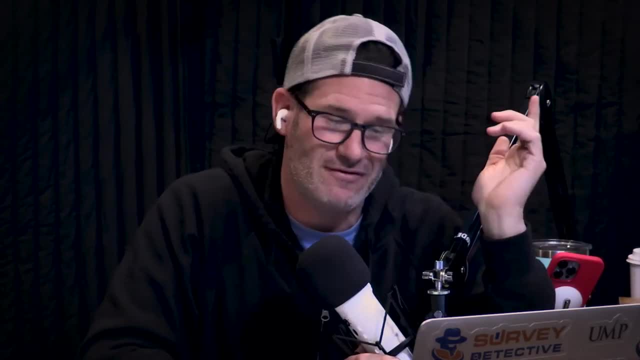 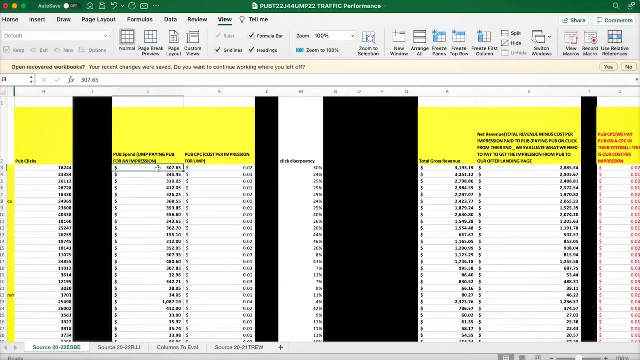 don't need me, You don't need anybody, You're not dependent on anybody but yourself. So when you understand this stuff, boom your money right. So I'll walk you through this a little bit. So pub clicks here. Right here is the spend that we have for getting those clicks right. So 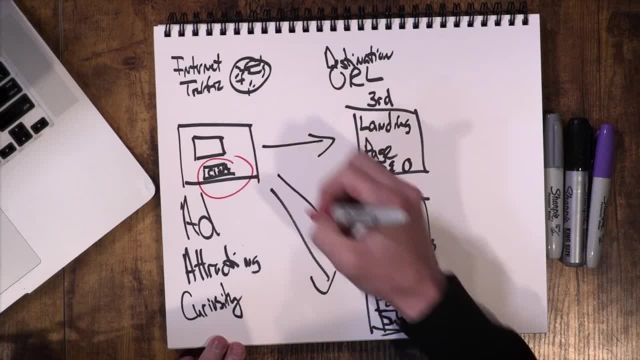 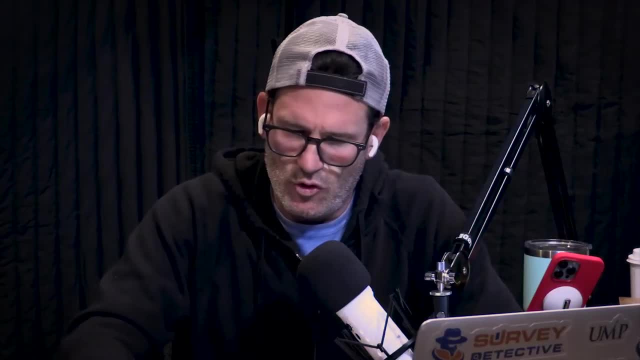 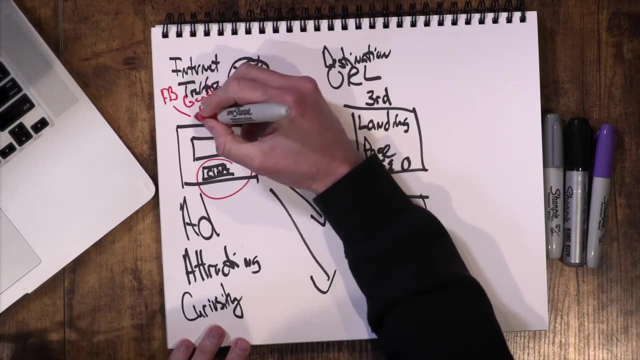 we're talking about the clicks here, right, So here's the click, right When somebody goes right. So internet and traffic. So let's say, Facebook, Google websites- right, They're all going to get you traffic. You're getting your ad in front of you. 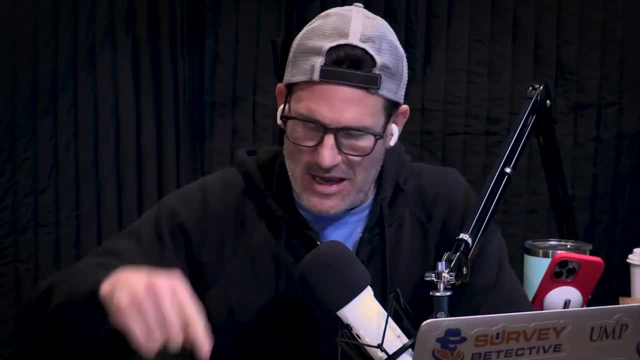 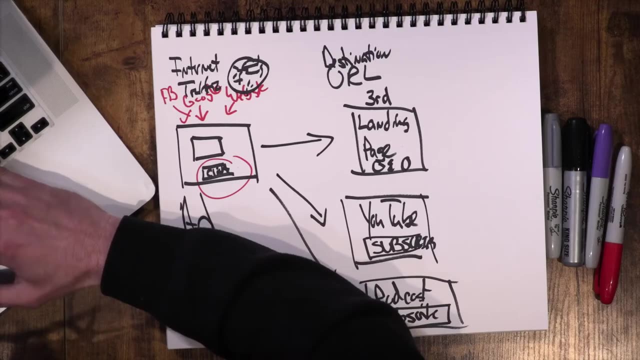 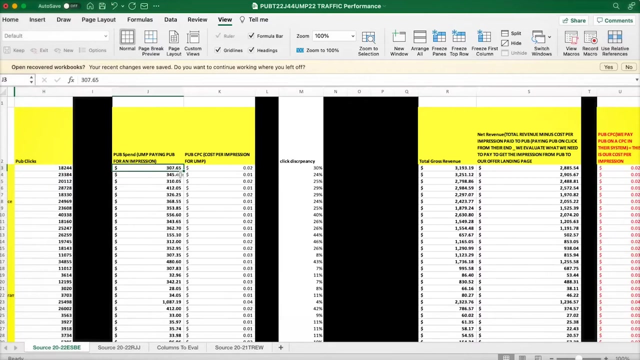 Of that traffic, that person that you're looking for And we're looking for a click. That is our goal, Our click right here And we're paying on a click basis, right. So 18,240 clicks right And we're paying $307.65.. So paying a pub for an impression. 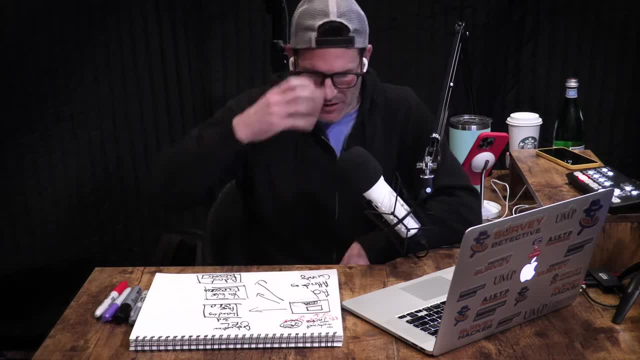 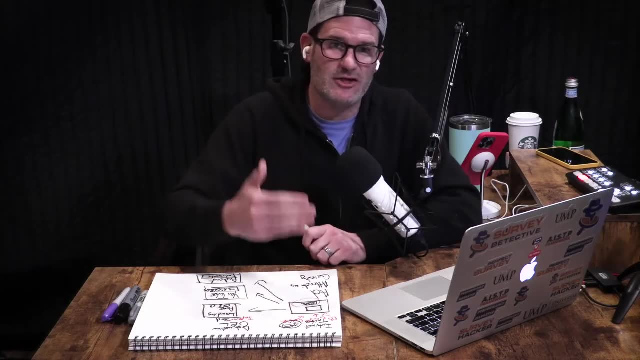 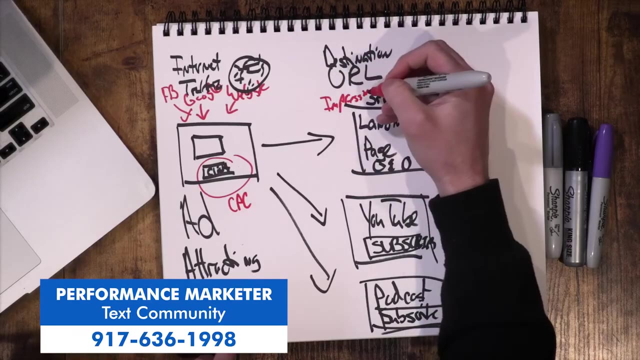 right. Well, what does that mean? So when you're paying for a click here to us, it's an impression To the person that you're getting the traffic from. you're paying on a CPC, right, But from here we're looking at it on an impression. So I like to look at revenue per impression, RPI, right. 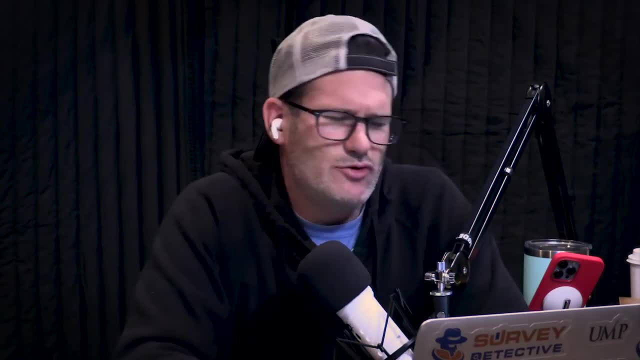 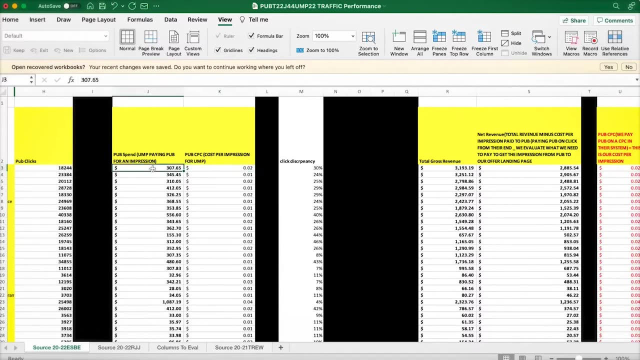 What are we paying to the partner? right now, It's two cents, right? So we're paying two cents. a click, at 18,240 clicks, We're paying $307.. And here is the click. So we're paying $307.. And here is the. 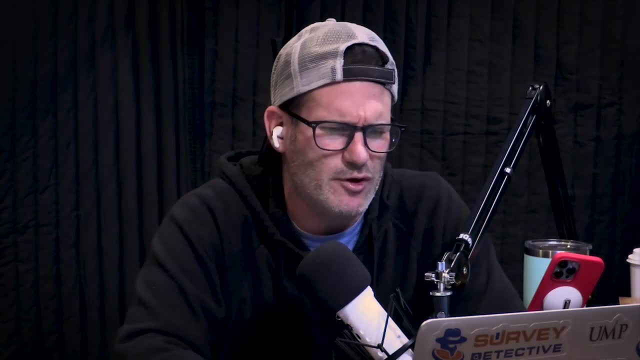 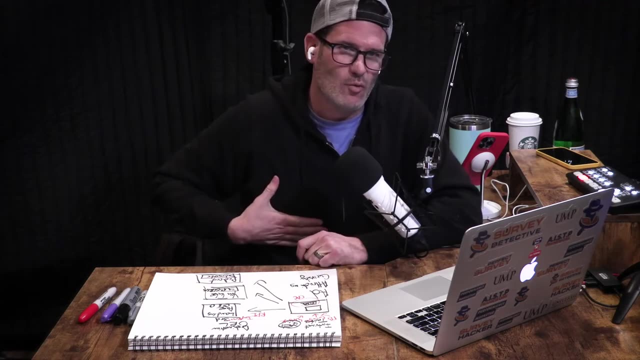 something that we look at, which is click discrepancy. I won't go into too much detail here, But ultimately, what is the partner showing on how many clicks they got us versus what is my system showing me of what we received on our pages here, right? So you know, discrepancies are big. 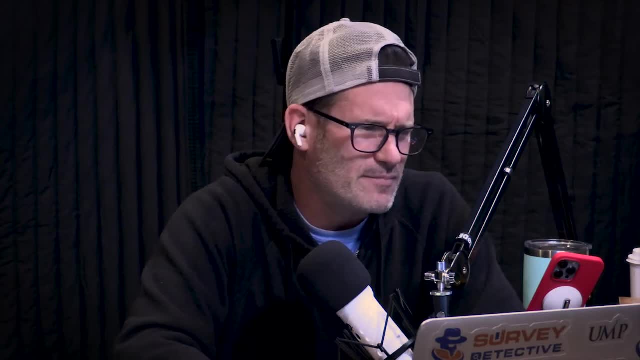 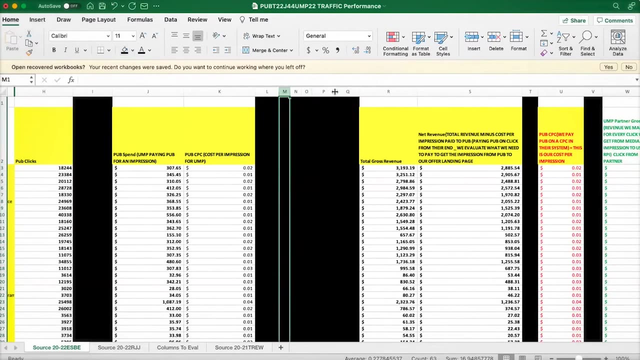 but it's not really important for this. So let's just get rid of the noise. All right, we're closing this down And I black things out just because it's noise for you guys. A lot of stuff here is not relevant. 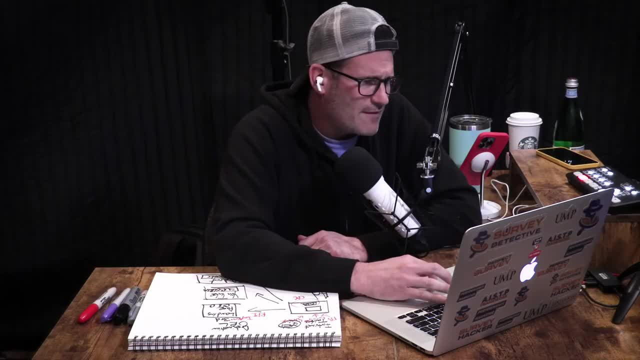 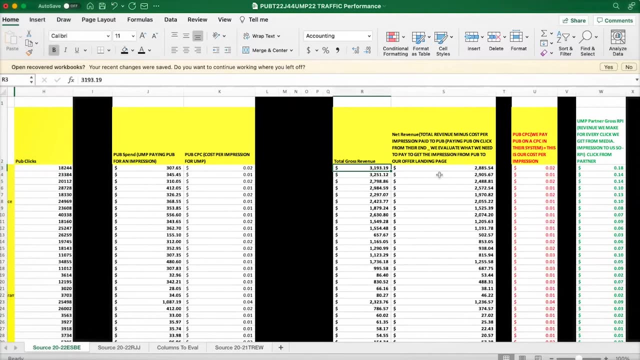 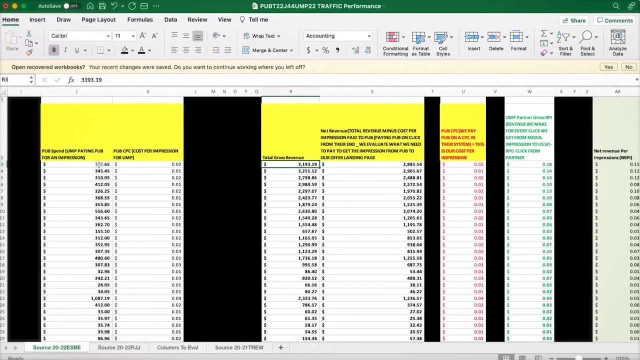 I want to keep it super simple to show you guys how to do this. So, on this 18,244 clicks, we generated $3,193.19, right. So the net revenue here is $3,193 minus the $307 that we paid to get. 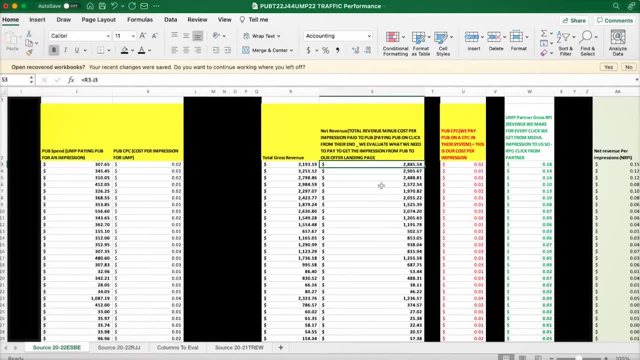 those clicks to equal $2,085.54.. Woohoo, baby, right, You're psyched, You're killing it. right, The pub, CPI, the CPC here of what we have. this is what we pay the pub in their system. This is on our cost, per. 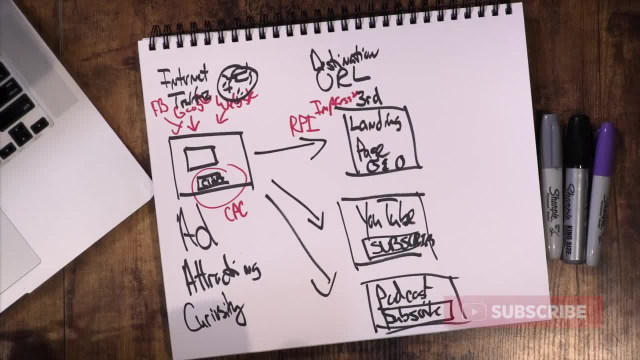 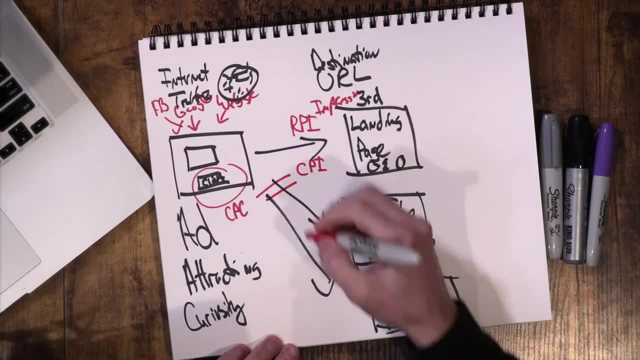 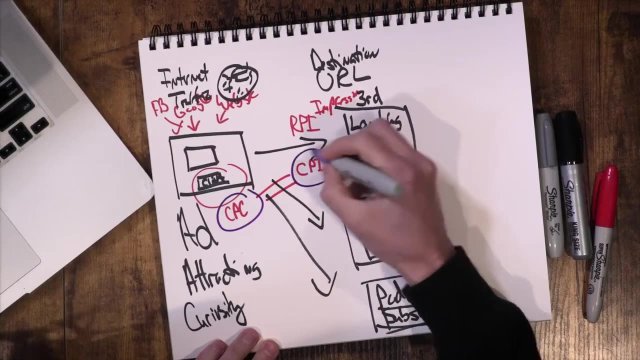 impression, right, So we're looking at revenue per impression. The CPC is really our cost per impression, right? They equal the same thing. It's the same thing here, right? Let's get some other colors here. So same thing, right? So the CPC is just what you're paying. 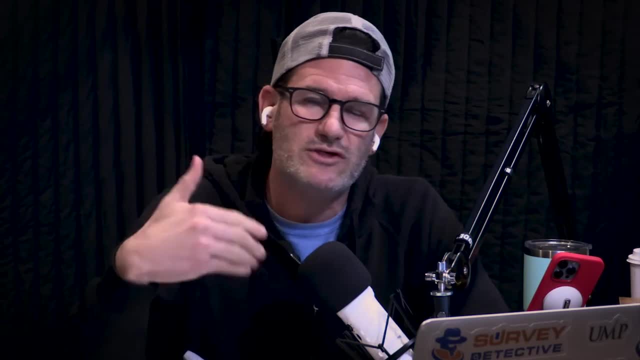 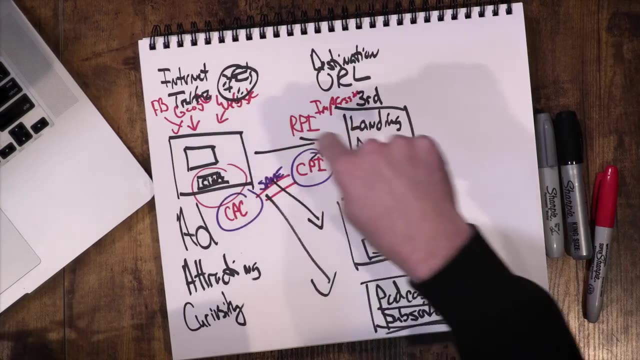 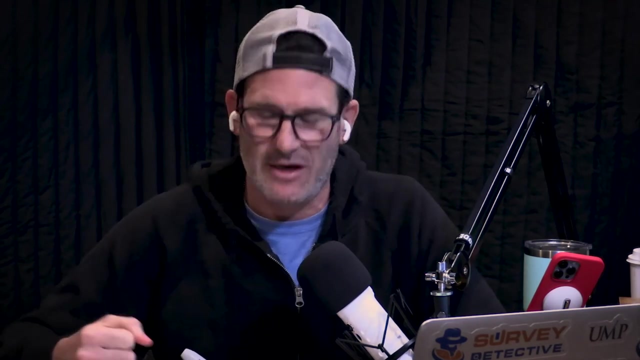 Out to the partners. But when we're evaluating traffic, we need to know what is our cost to get that impression, to get that person from wherever they are on the internet over to one of our pages. That's our goal. Our goal is to get people off of other platforms into our world, right? That's why 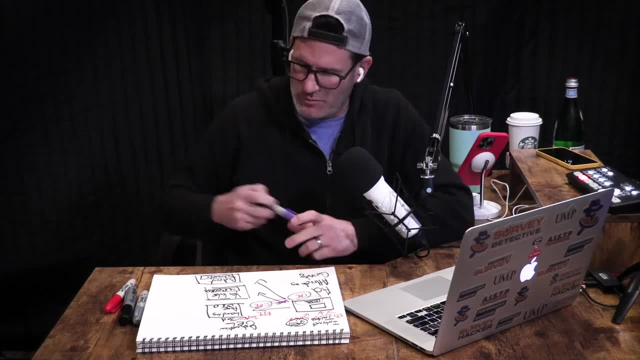 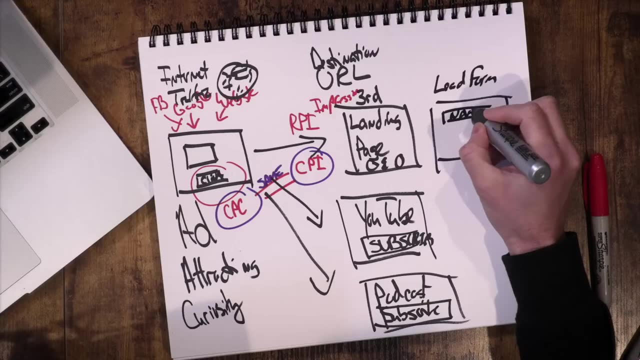 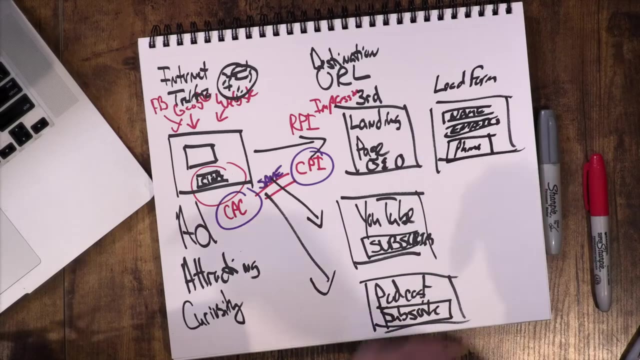 we want to capture data right On a landing page. we could have some lead forms, right. So, like a lead form, you know name, email, maybe you need phone. whatever, that is right. Why is someone going to give you that Well? 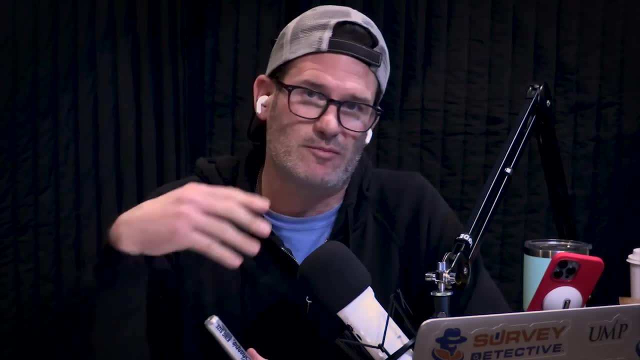 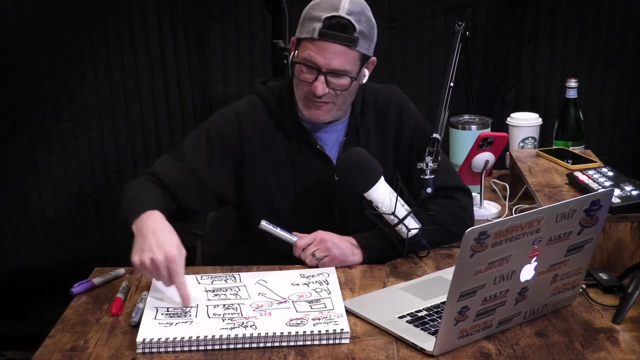 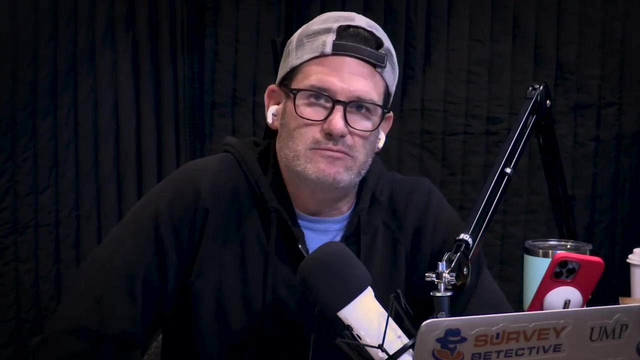 you got to give them something that is interesting, right? That's why you either may have something on there that you're giving away for free, that is of value to the person, and you're trading them their information for your free: 10 secrets on how to consolidate debt, right? Whatever that secret. 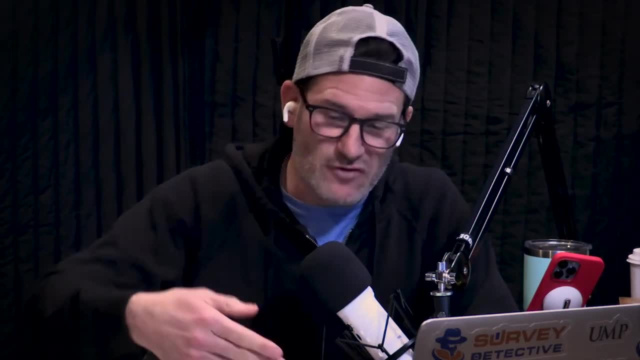 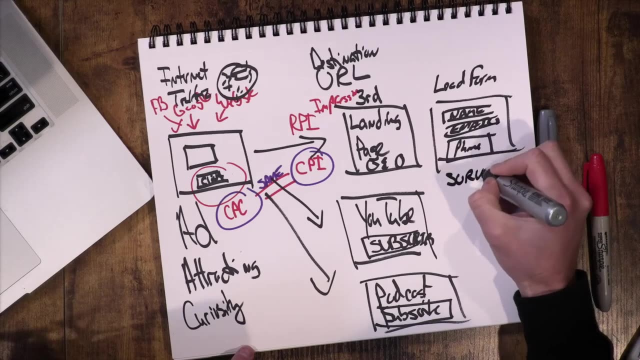 is, whatever that value is that you're doing right? That's what you're doing. That's what you're doing right And we could talk about that. We've done it before. lead magnets, whatever right. Another way to do it is we can do it driving them to a survey, right, And here we have our headline. 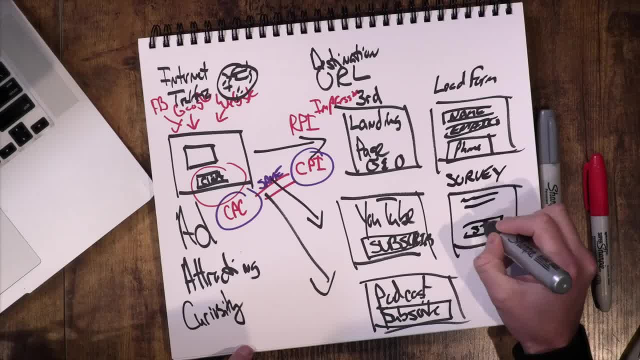 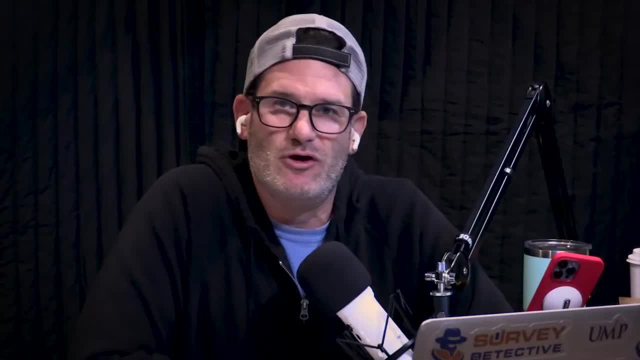 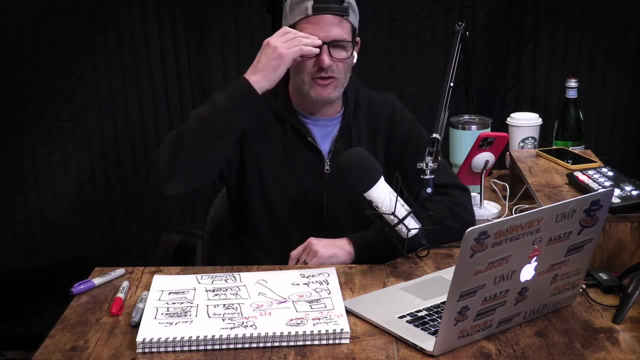 that's curious based and our start page, because we're driving people somewhere and we don't want to just ask them to give us their information right away. We just you know, you want to talk to them, You want to understand them, You want to try to give them something of value. 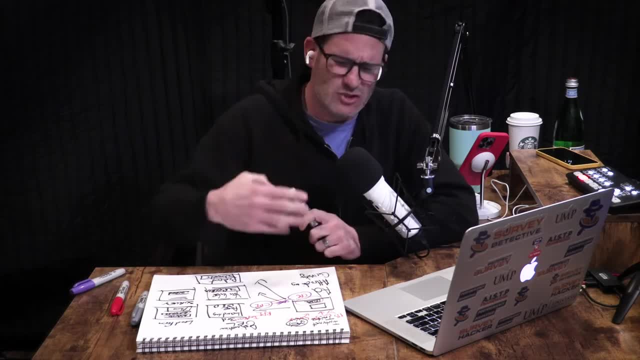 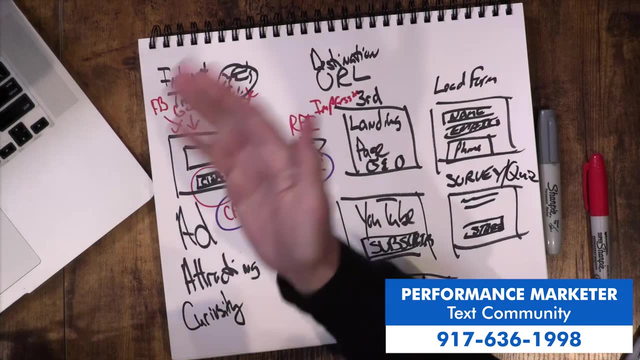 right, So you create some curiosity. The beauty of like surveys, quizzes, right, It's the same thing. Quiz is that you're allowing somebody to come in and learn something about themselves. You're getting them curious about whatever. it is right, So it's a. you know what type of home is. 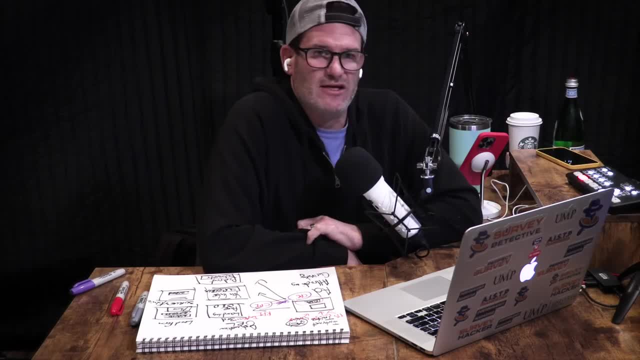 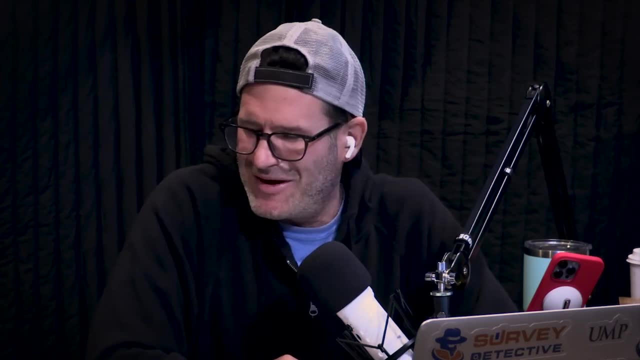 right for you Five mistakes people make when they're consolidating their debt. you know things like that right Now, and that's interesting, right? There's four types of parents, Which one are you? You know, I'm learning some of myself, right, And you're making that. 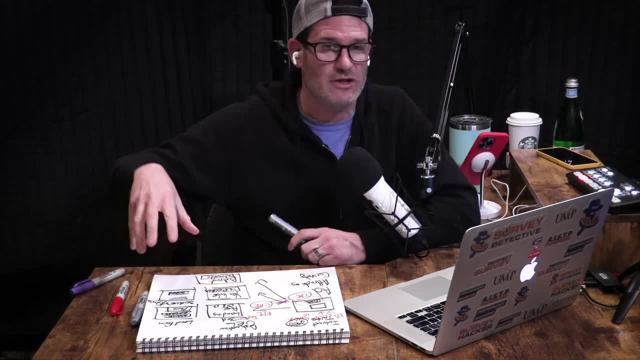 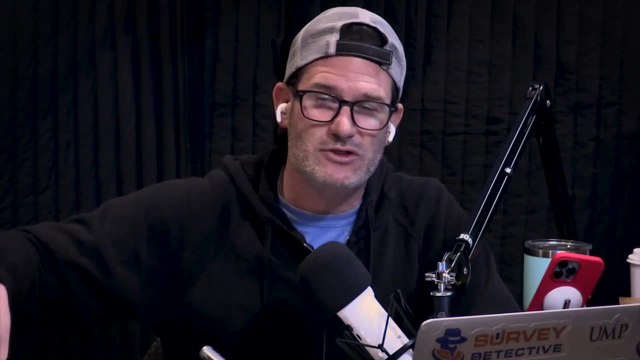 promise You're going to tell me what to do. You're going to tell me what to do. You're going to tell them at the end. So then you get people to answer all these questions that are really awesome. at the end You get there and then to give them the results you make them give you something in. 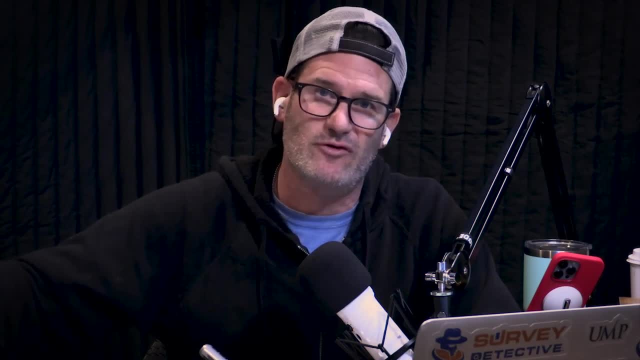 return right, You're giving them something of value, So then they can give you their name and email.